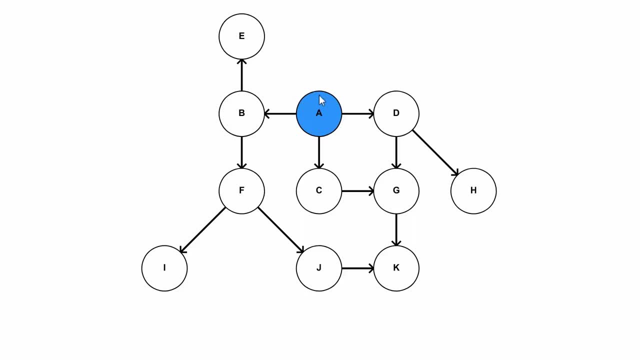 for search. So what you're doing is you're running depth for search And then when you're done with the function that you're running on a particular node- so when you're done with a node, basically you add it in reverse to a list. So we're going to do that down here. So we start with A. 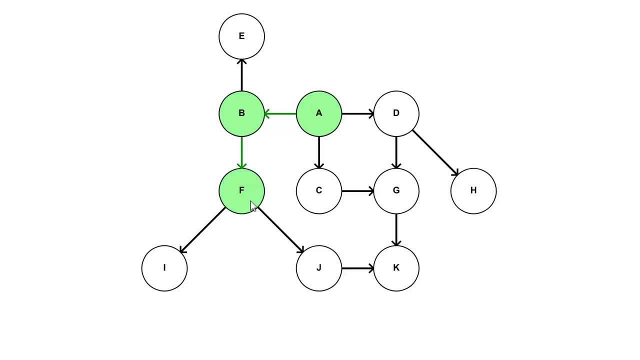 and then we just do a depth for search. So we go to B and then F and then I. So I is a node that we're actually going to return out of. So we're going to be done with I now, which means 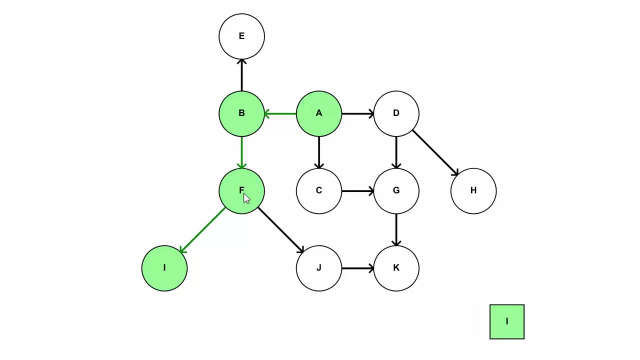 we're going to add it down here, And then we're going to continue here with F, And now we're actually done with K, So we add it here. Then we're done with J, because that was its only child, And then we go to F and we're completely done with F. now We have explored all the children. 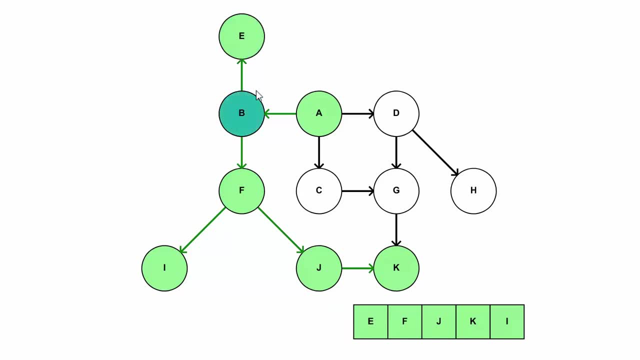 So back up to B, explore E, done with E, and now we're fully done with B, And so we can continue down to C. G points to a node we have visited, So we don't do much there. And then we're done with G and now done with C And still not done with A, because I still have. 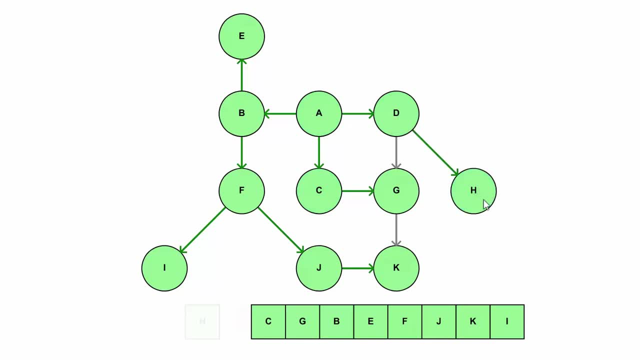 children we haven't explored. But now we go into H, which we are done with, And we're done with D, And now we're fully done with A. So this is a sequence where we have all the kind of dependencies. So A is a dependency. 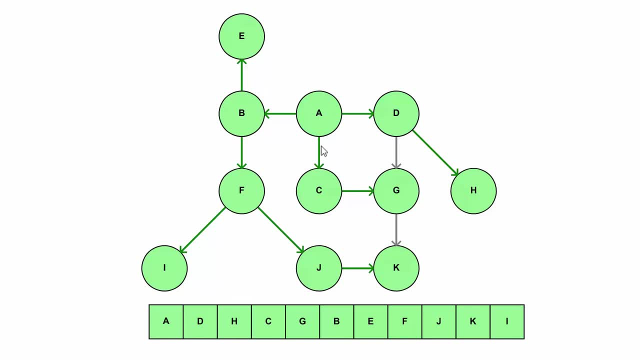 It's a dependency for everyone. So that's first. But yeah, let me visualize this in another way. So if we start with A, here are its children, And so now I'm just going to follow the sequence that we have made, So then we can do D, because it only has a dependency of A. So that's perfectly. 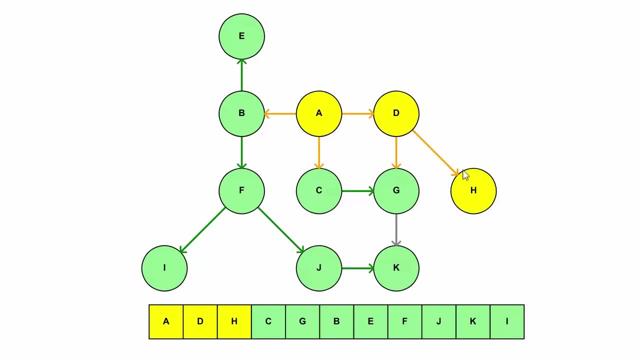 valid for us to do. And then now we can do H, which has a dependency of D And C, still perfectly valid G, And now we can go to B And E And F And J And K And I, And none of these had dependencies that 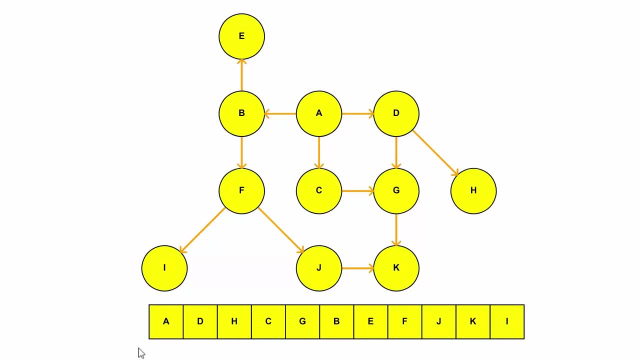 we haven't colored yellow, So this sequence is correct. It's one of many With depth of search. since it is a bit random, you can have multiple valid sequences, But that was topological sort.